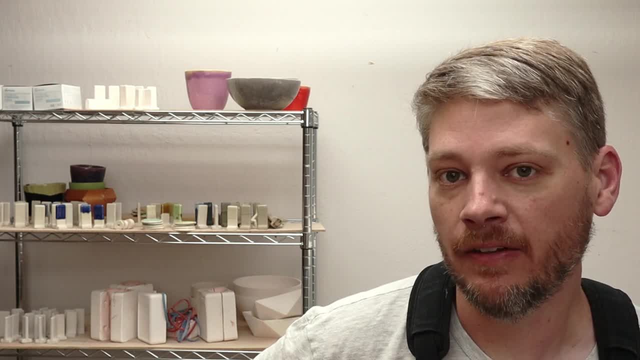 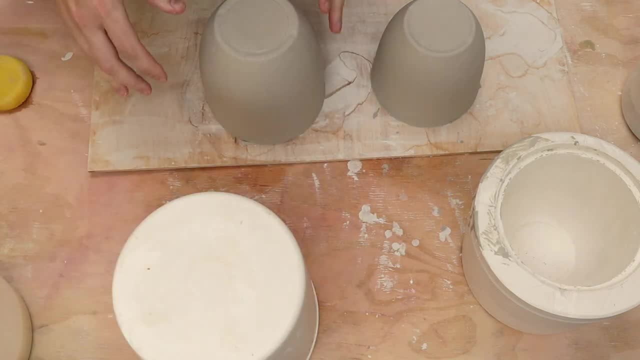 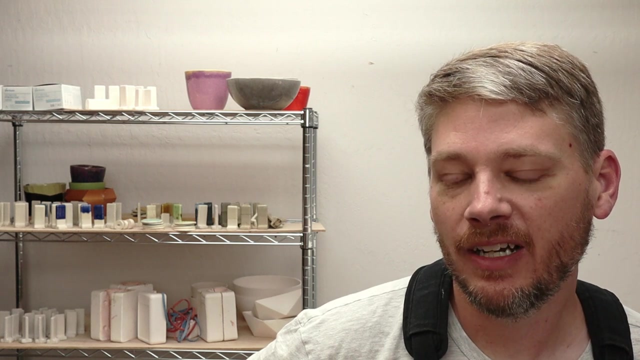 Hi, I'm Kent. In this video I'm going to go back to the basics of slip casting. Life has been a bit busy recently so I haven't had a chance to do pottery or the associated YouTube videos. So to warm back up, I just want to do some basic pots. 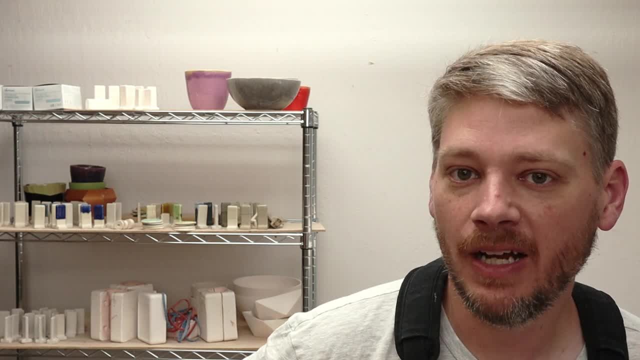 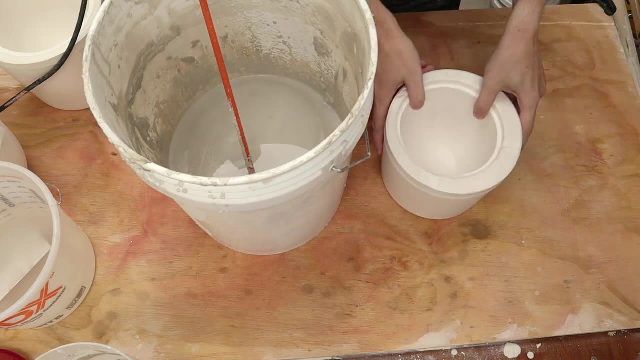 I have two new plaster molds that I just made and I'm going to slip cast a few pots To make my pots. I am slip casting, So for that I need some slip, which I have here, and some plaster molds which I've made. This here is my slip. It's been sitting for a while. 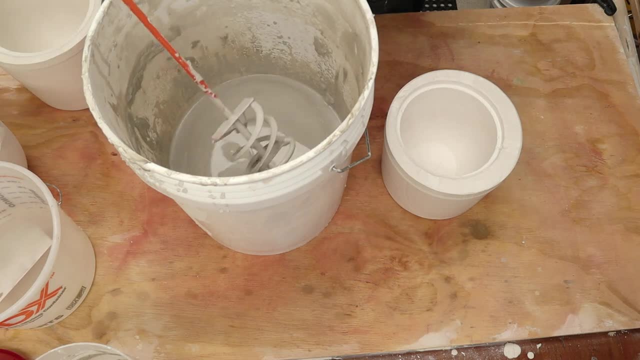 and I just mixed it up here with my drill and I have this paddle attachment here. The consistency is looking good, Nice and fluid, so I don't think it's lost too much water. And here is a mold. This is actually a new mold I just made the other day. 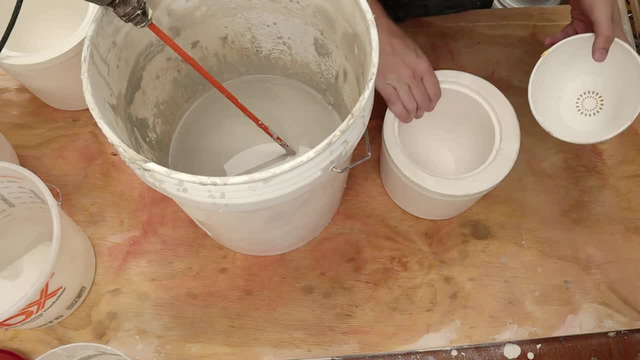 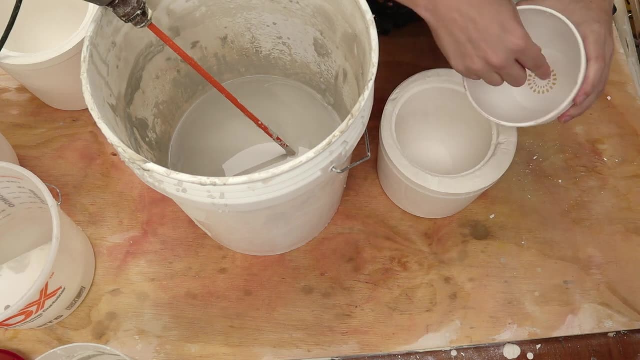 I've been experimenting with ways to make these plaster molds, So this one here is actually from a plastic planter I bought on Amazon. I 3D printed a bottom so that I could deal with all the holes. I also 3D printed a top so I could form a lip- The top part I was hoping to reuse. It worked okay. 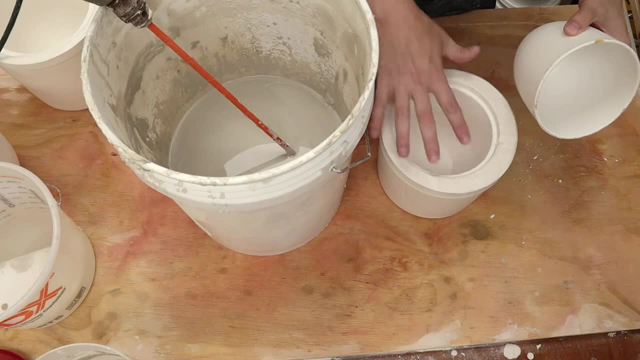 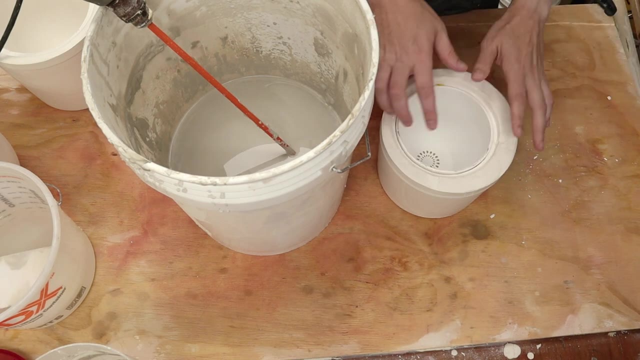 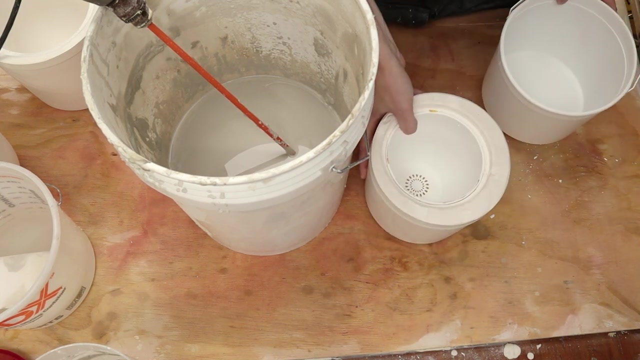 but it failed when I was pulling the planter out of the plaster. I don't think I have enough of a lip. I also have a few bubbles that formed, And in the outside container I just used a tub, So it was basically formed like that. I popped it out. 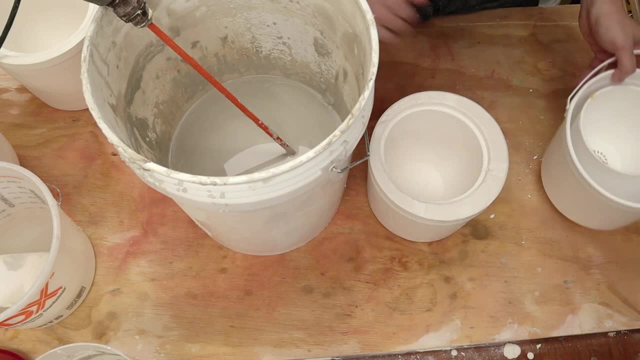 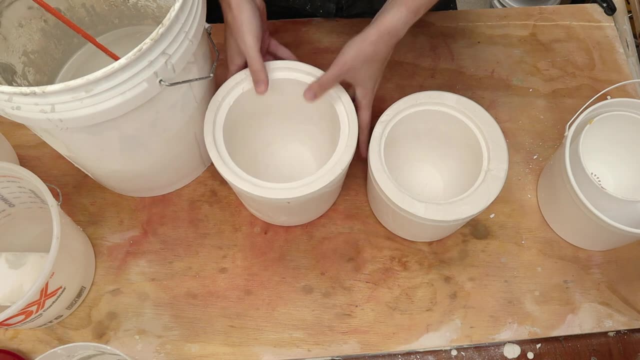 I made sure to have mold release on it. Then I have this mold here and I actually made a second one- It's hiding off to the side here- And I made a second one here out of a larger planter. So these are the two molds we're going to use today. This will be the first casting in both. 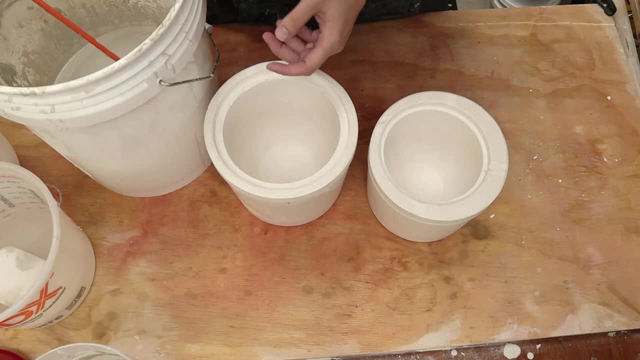 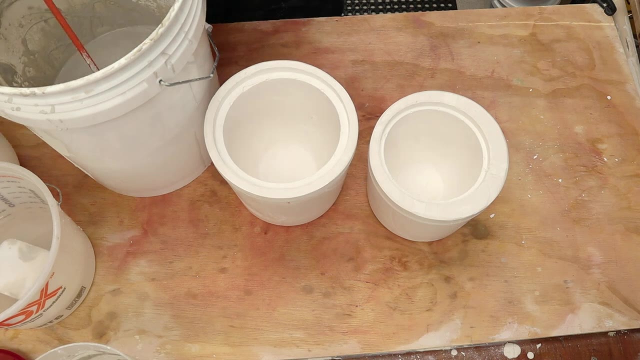 of them. This is a five gallon bucket, so when it's full it's crazy heavy. but right now I don't have but maybe a gallon left, so I think I can just pick it up and pour directly into these molds And we just pour the slip in. 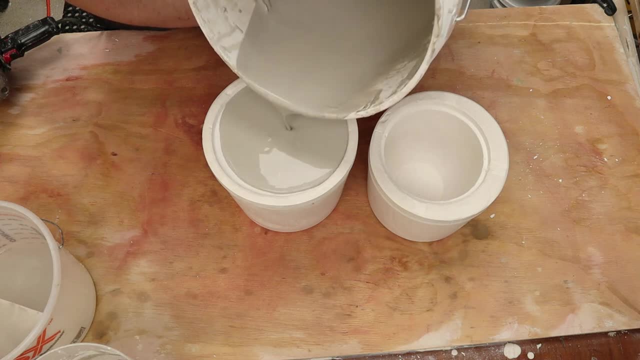 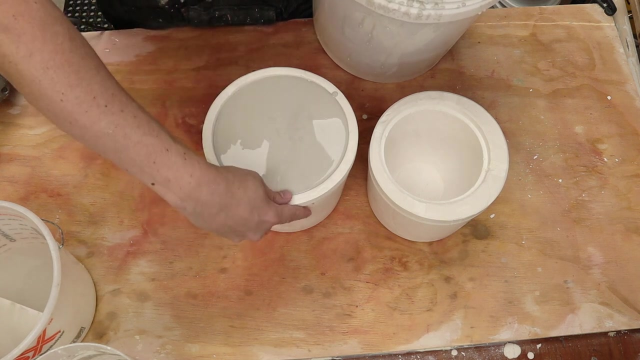 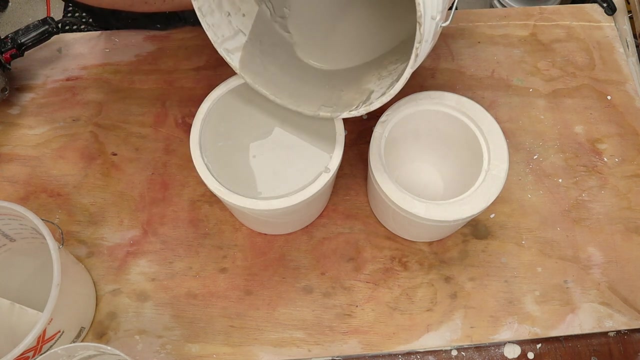 I'm going to rub the bottom of the container in here, So this slip here is above the top of the finished pot, so that gives a little bit of extra space for the slip to sit As the water gets sucked in the plaster it'll actually go down a little bit. 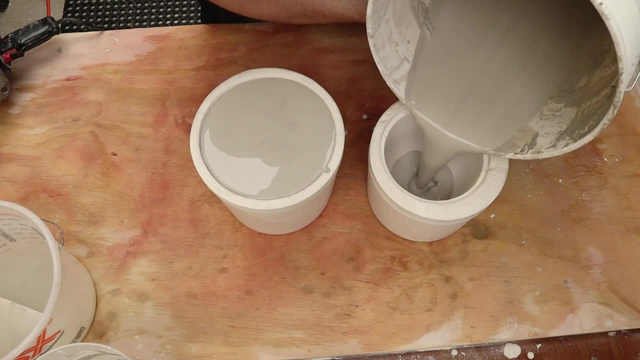 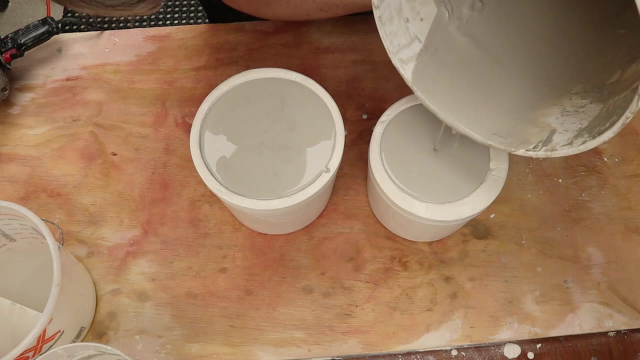 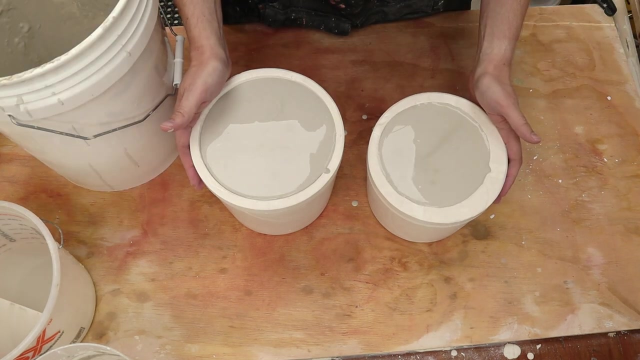 See if you can put a little bit more in without going over the edge, And it looks like I have just enough. slip just a tiny bit left Next up. these just sit for a while and the water will get sucked into the plaster and 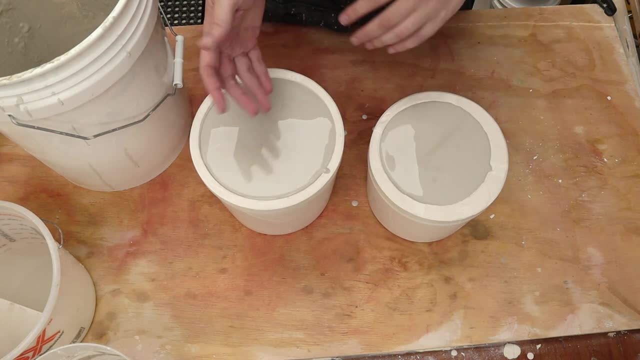 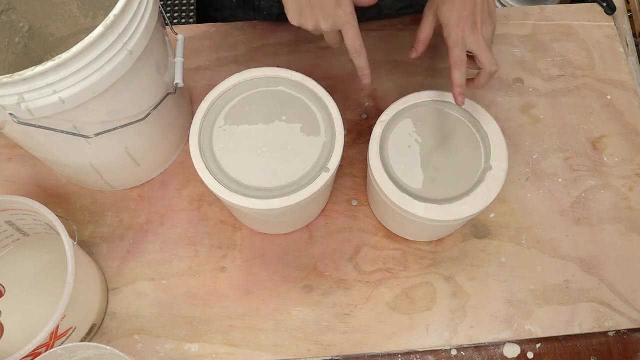 form the pot around the edge. So we'll come back to it in a little while and dump the slip out. So these have been sitting for a while and you can see the level of the slip has dropped down. It looks like it's getting close to where the shelf is. 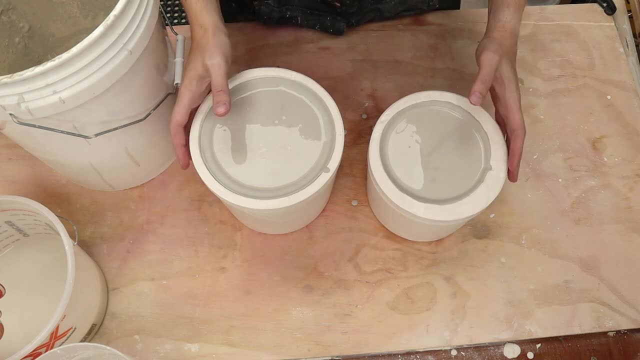 These are obviously the first time I've used these molds, so I'm not too sure exactly when I should pour out the slip, but we're going to give it a try right now. So there's the bucket and we're just going to dump it in. 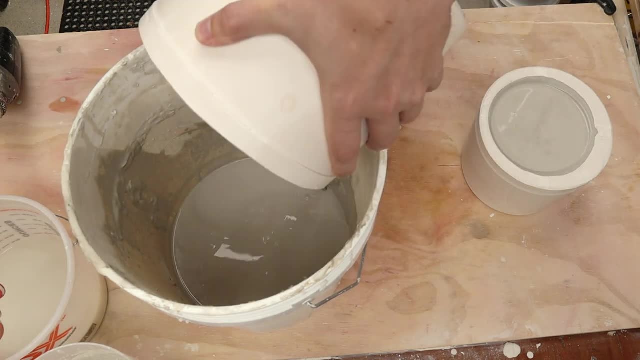 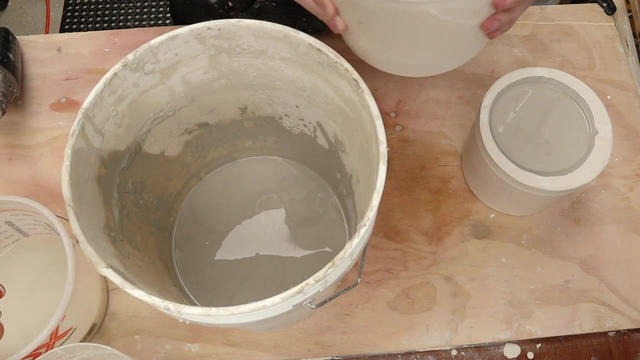 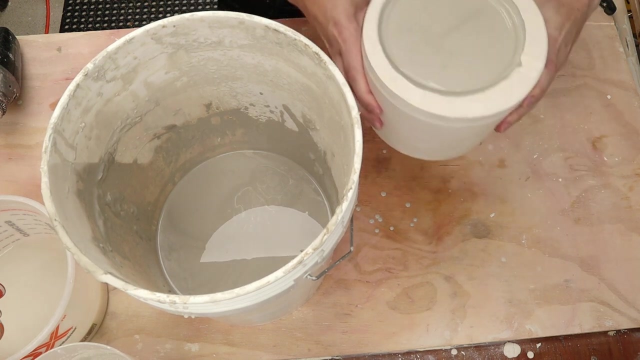 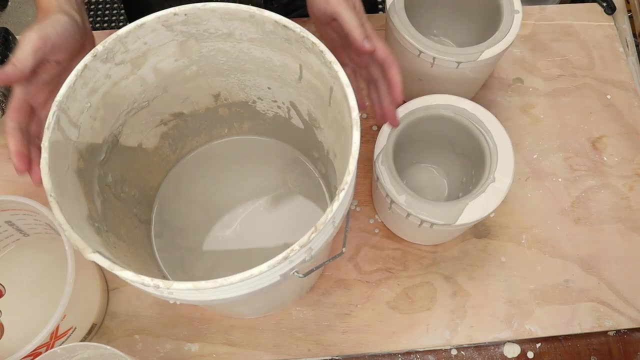 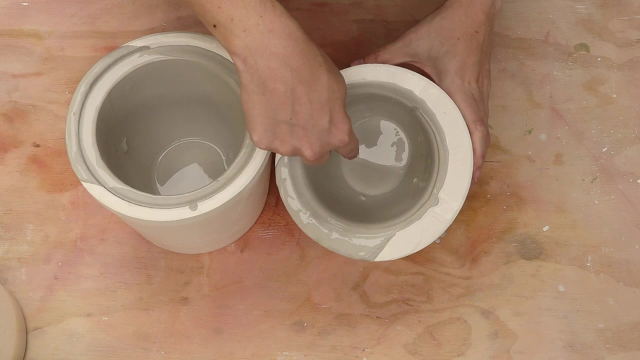 Heavy. All right, that worked out pretty well. I need to drain a little bit more, but let's do the next one. All right, so we should be done with the slip for now. There's still a little bit of excess slip here. I need to flip them over and let it. 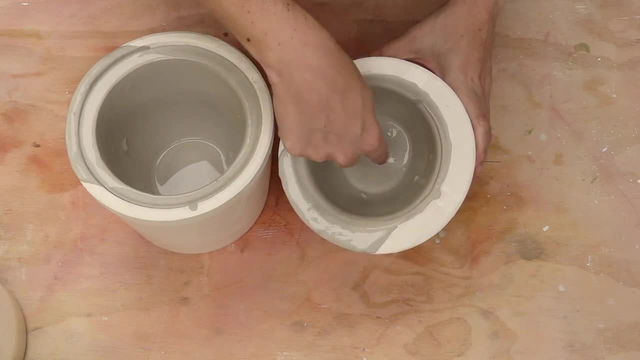 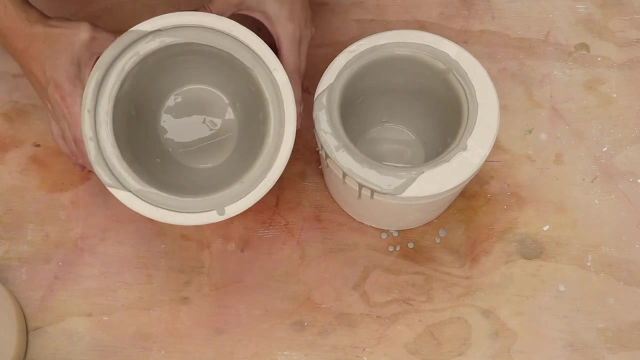 drain the rest of the way. You can also see a few chunkies in the side. That's because my slip has been sitting and I didn't run it through a sieve And there's that one. So let me flip these over. drain out the rest of the slip. 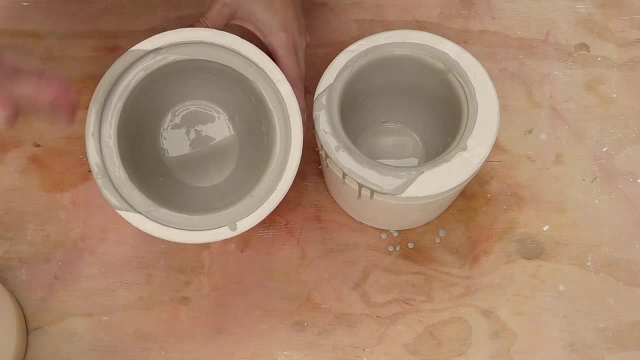 And let them dry. All right, All right, Let's flip them dry so that we can then pop them out. These have been upside down, propped up on this piece of dowel for a while so that at an angle can drain out. 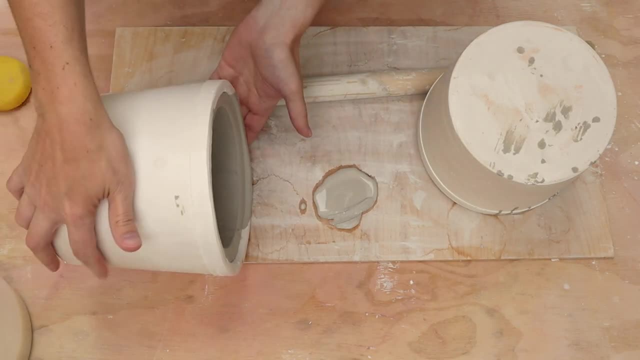 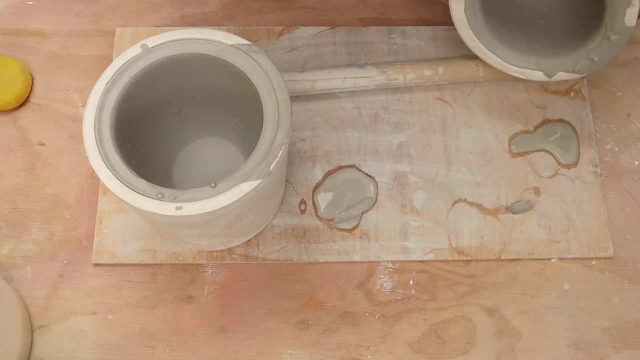 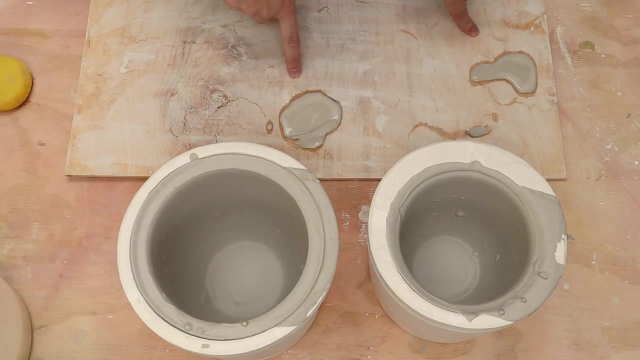 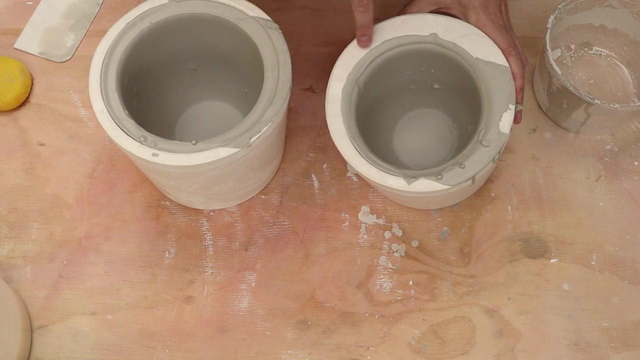 Let's check them out. There's all the excess slip That looks pretty good. Cool same thing. The slip here on the board I can reclaim and use at a later date. If you look real closely here you can see it's starting to release from the sides.